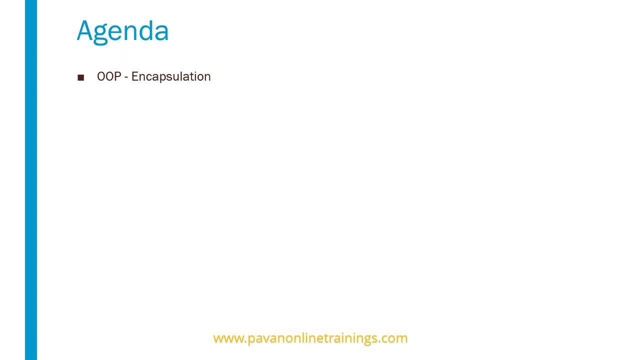 hello everyone, welcome you all. so in this video I'm going to explain about encapsulation in Python. encapsulation in Python. so let us see what is encapsulation. so what is encapsulation? so in an object oriented Python program? so you can restrict the access to the methods and variables. so this can. 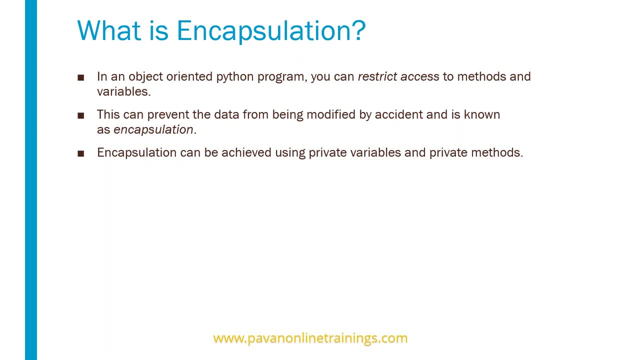 prevent the data from being modified by accident and is known as encapsulation. and encapsulation can be achieved using a private variables and private. so encapsulation means we can just wrapping up variables and methods, we can just restrict the scope of the variables and methods. okay, that's called as an. 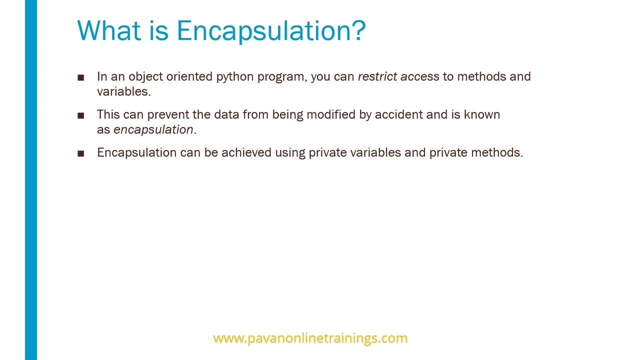 encapsulation. so this can be achieved by specifying a variable or methods are private, but how we can specify them as a private. so in Python we can specify a variable as a private. so in Python we can specify a private. so in Python we can specify a variable as a private. so in Python, in. 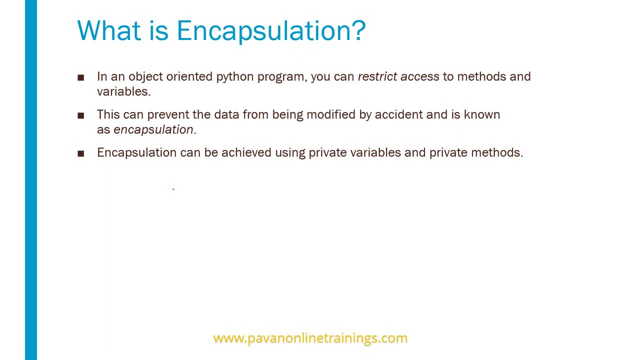 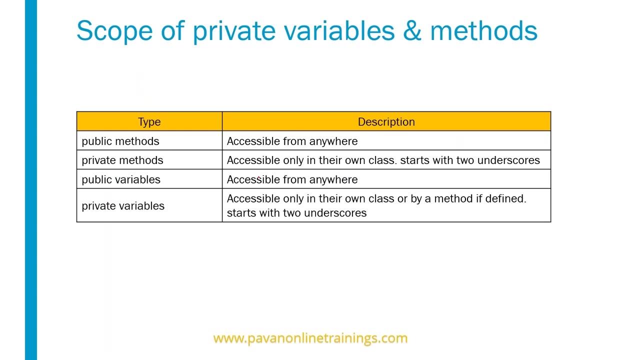 other languages we have a private keyword, but here we can specify method or variable as a private by specifying the two underscores: two underscores in front of the variable and in front of the method. now let us see how we can do this. encapsulation with some examples. okay, now, as I said, encapsulation can be. 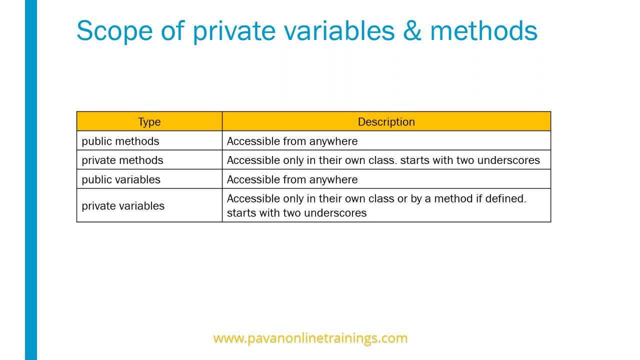 achieved by using private variables and methods. right now, when you see if I create a variable or method as a private and what is the scope level, suppose if you have a methods, public means, if I don't say private, okay, if I don't specify the underscore, private is nothing but underscore, underscore in. 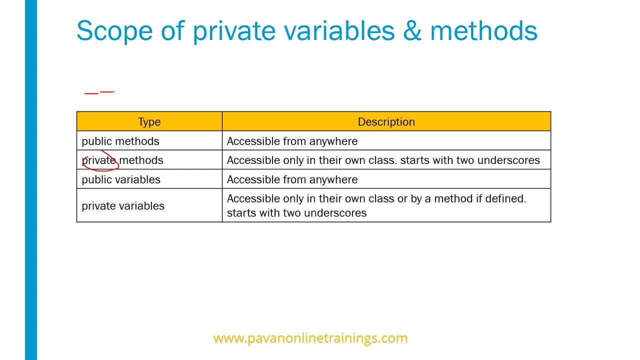 Python format. if you specify any variable or method is a private, we have to say underscore, underscore. if I don't specify underscore, underscore, that will be treated as a public method. okay, so public methods means general methods accessible from anywhere. we don't have any restriction for that, but especially for private methods accessible only. 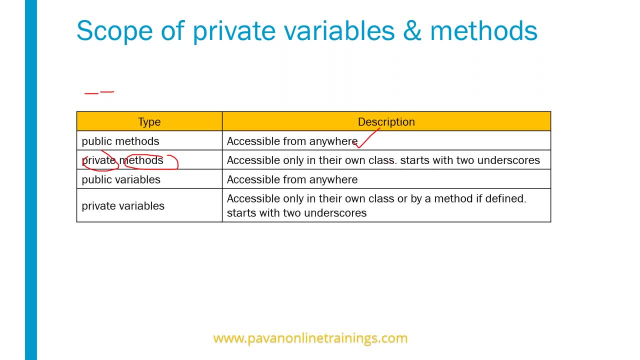 in their own class. okay, and these private methods will start with the two underscores: underscore. underscore and private methods we can access only within the class. outside of the class we cannot access. similarly, public variables can be accessible from anywhere. that means public. we don't have an issue. we. 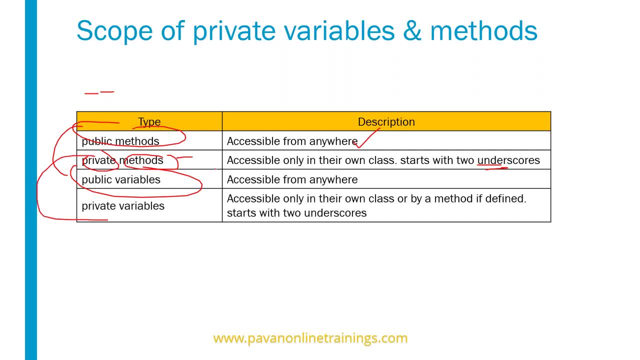 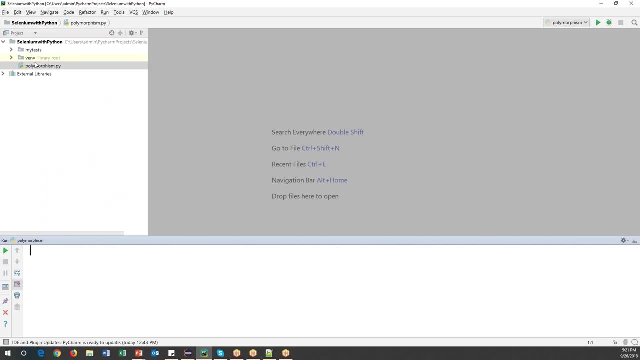 can access to any ways, only the private variables and private methods. private variables, private methods, can be accessible only within the class, only within the class. now let us see how we can do this practically. let me open my patron. so here I will create a new file, new Python file. I will name it as an. 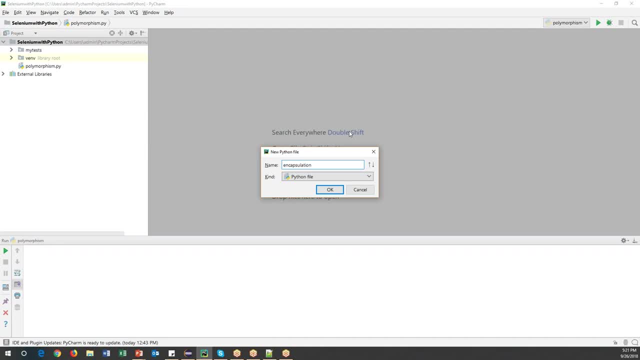 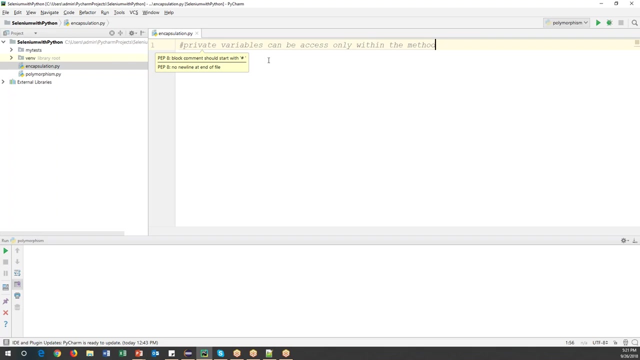 encapsulation, I will name it as encapsulation. so now here: encapsulation we can achieve by using private variables and private methods. so let us see one example. so either say: first point: private variables can be accessed only within the method. so private variables is a first exam. so private variables can be accessed only within the method only. 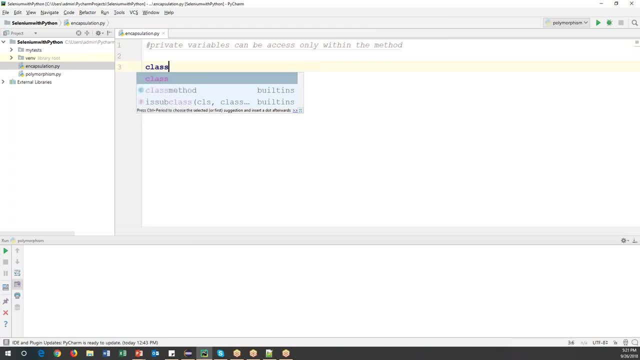 within the method. now let us see how we can do that. let me create one class. I will name it as a my class, right? so in this class I will create a private variable. so how to create a private variable: underscore, underscore and variable name is, let's say, a, and I'll put some number here. this is called as a. 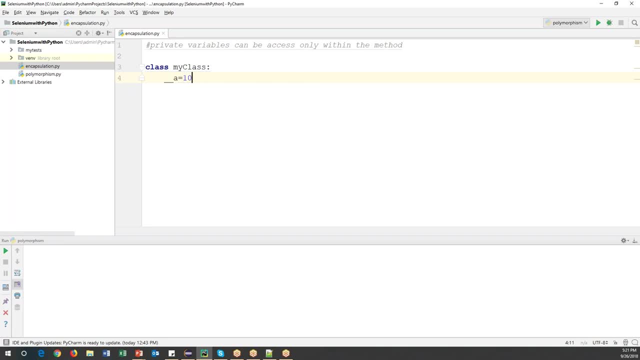 private way. so what is the scope of this variable? only within the class, only within the class. now, along with this variable, I will also create one method within the class, let's say this diff display, and here, in this method, I will just print the value of this variable. now, here how to write print statement a. 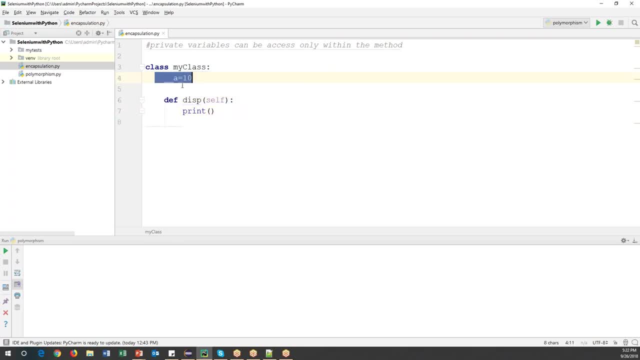 print print. so how we can access the class variable, how we can refer the class variable by using self, the keyword rate cells, dot. what is a variable? everything underscore, underscore, a. because it is a private variable, we have to call always underscore, underscore. okay, so now this will print the value of this variable. so 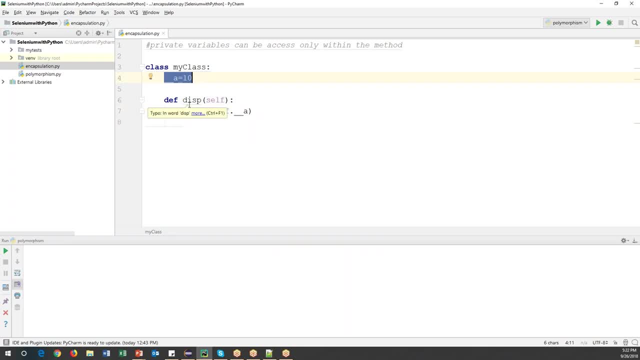 why we have specified self here, because this is a class variable. if it is a local variable, we can directly print here, but it is a class variable, so that we have to use self keyword now here, after creating this method, let me create an object for this class. OBJ is equal to. I will create an object for this class. 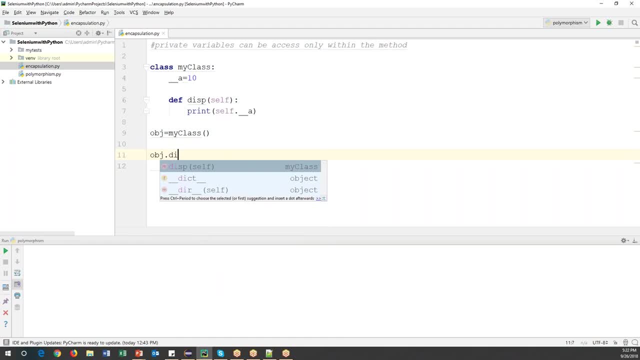 now observe this: I will just call this method by display method: OBJ dot. this plane, OBJ dot display. so we print are not. so it should be by, because when I say over this William inter, it will call this function or method internally we written print statement I'd. so this method is a part. 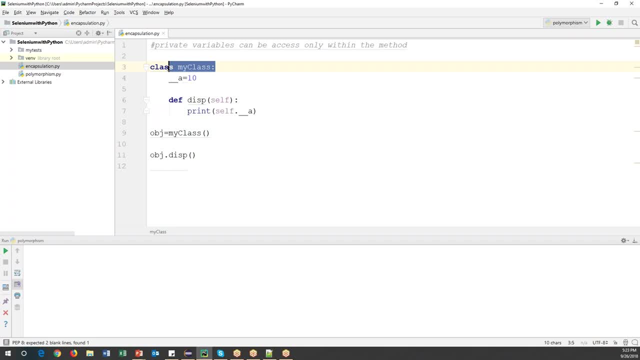 of this class are not, so this method is also part of this class. so So this variable can be accessed within the class. So method is also part of this class. So this method is directly able to access this variable value. So we can just run this. you will get exact value. 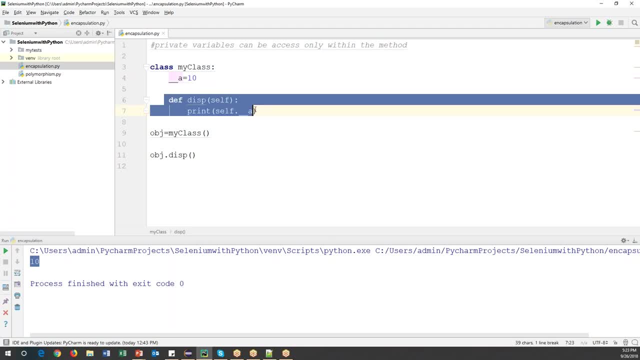 So here we don't have any problem because this variable is in the class method is also in the same class. Now I have called this method using an object, So it is able to call perfectly. right now I'm trying to access this variable outside of the class, outside of the class. how we can. 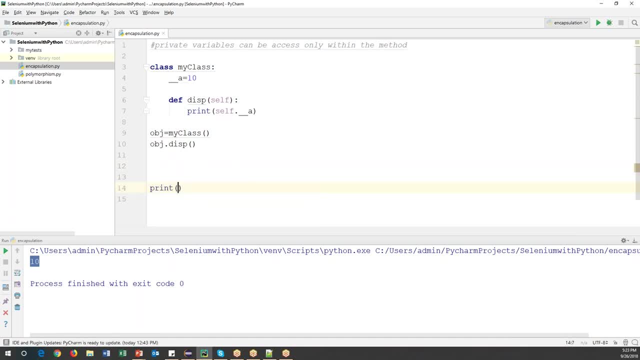 access this variable outside of the class. So I will directly use print. and which class? this method? this variable is created inside the my class, right? So how we can call this? one class mean, let's say, my class, my class dot, underscore, underscore a. So this is how we need to call if it is a public variable. if it is a public variable. 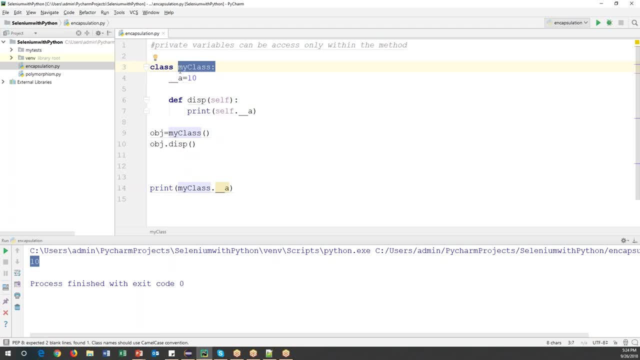 we don't have any issue. So we can directly access this variable by using this class, all right, but because of this is a private variable, we cannot directly access this outside of the class. currently. we are in outside of the class, right? So my class is my class name. underscore. underscore. a is a variable name. 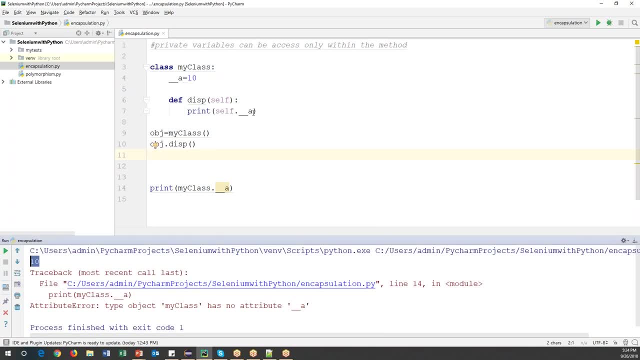 Now when I run this code, see now this value is provided by this one, but the second time in a call this it is giving an error. whatever it is giving attribute error type object: my class has no attribute underscore, underscore a: Okay, That means we are not able to access this. why? because this is a private variable, as 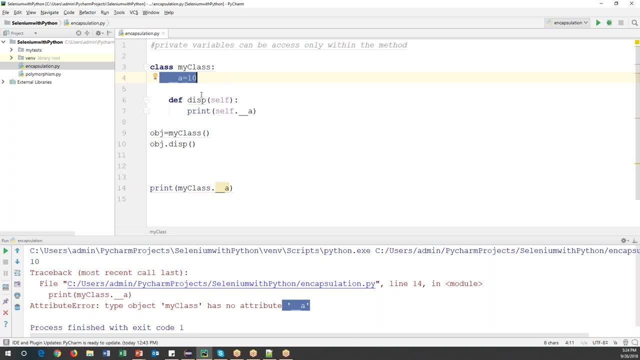 I said before, private variables are limited to this particular class, only within the class we can access. outside of the class we cannot access. So here we cannot, we cannot access because it is it is private variable. This is a private variable. how we can make it a private? with underscore, underscore, all. 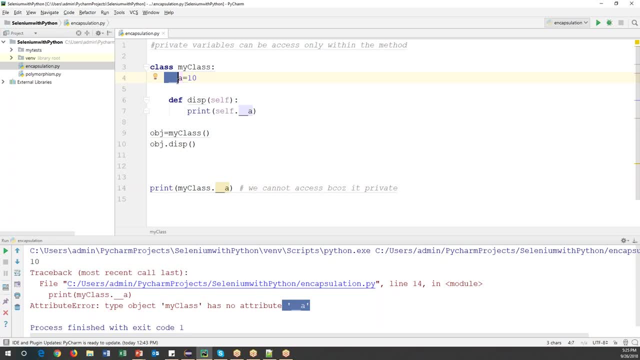 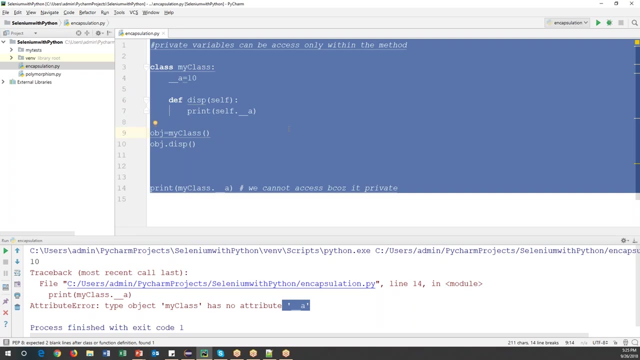 right, So? So private variable as underscore. underscore that will be treated as a private variable and that variable can be accessed only within the class. outside of the class We cannot access. right, and similarly, I will also show you private methods. So let me just remove this example. 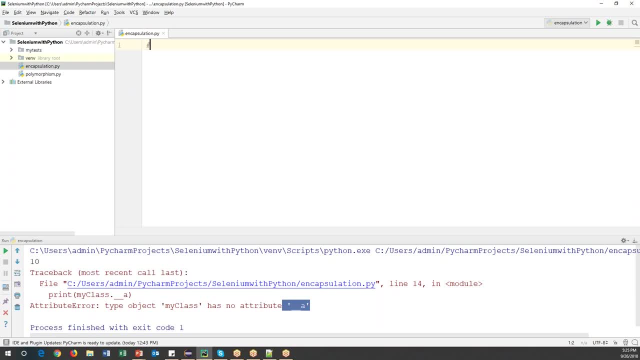 So I will create one more example. So this example I'll show you: private methods can be accessed only within the method. again, It's just like a private variables. private variables can be accessed only within the class. outside of the class We cannot access. similarly, private methods also can be accessed only within the class. 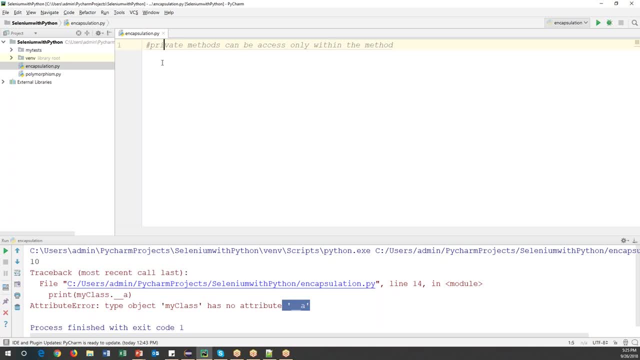 outside of the class We cannot access because that is a private. now, What I can do is I will create one more class. I will name it as a my class. Okay, This is my class. inside this, I will create one function, one method. def. underscore. underscore. how to create a fun. 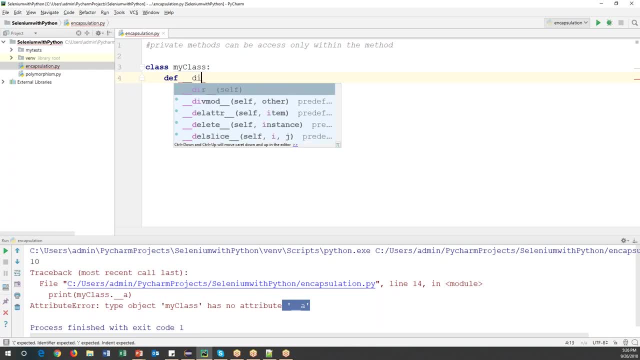 a method, private method, underscore, underscore, underscore, underscore. I will just say: display one, Okay, this one, and we will take self keyword and here I will just print: this is a display, one method, Right? So this is display one method. This is a display, one method. 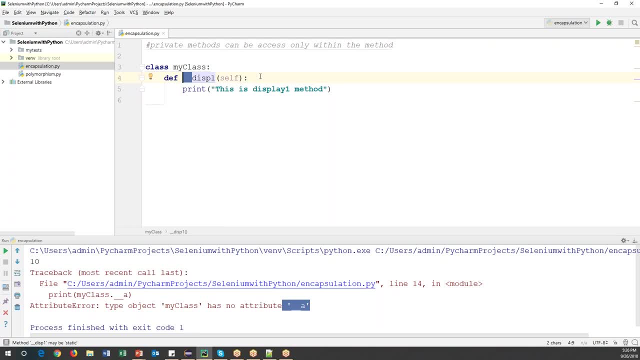 So as soon as I say underscore, underscore here, this method becomes a private method. Remember this. I'm just writing the comment. This is private method. This is a private method. This is a private method. Now, along with this, I will also create one more method that is a public, that is not private, because I need 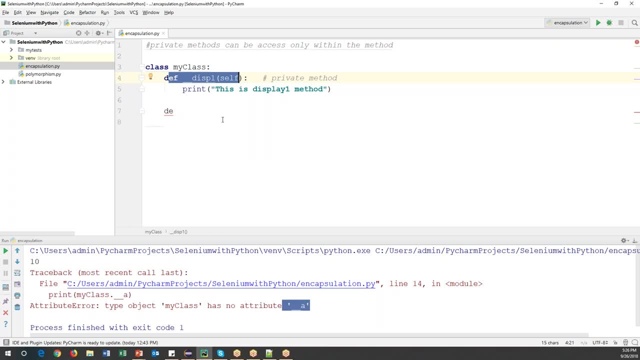 one more method to access this method, because this method we cannot access outside of the class. but how we can access this method inside of the class, at least we should have one more method which is public, and then we can call this method within the method. Let me show you. 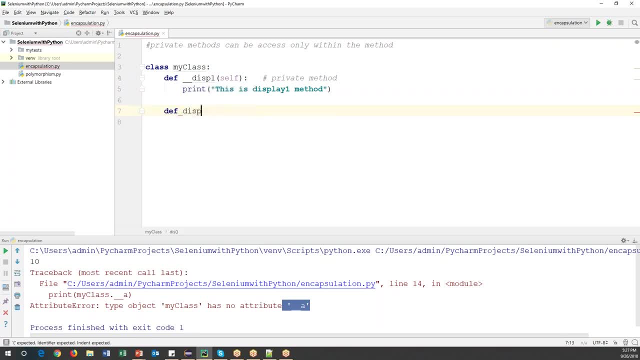 So here I will create one more method that say def display to this is not private method. Okay, So inside this method I will write some message And this is display. This is display to method. This is display to method. All right, 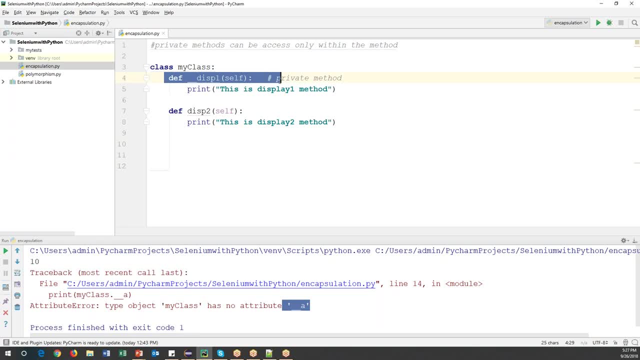 So now I just created some message. Now you can see here in this class I have two methods I have defined. the first method is completely private method, underscore- underscore I defined- and the second method is normal public method. But, as I said, this method can be accessible only within the class means I should have. 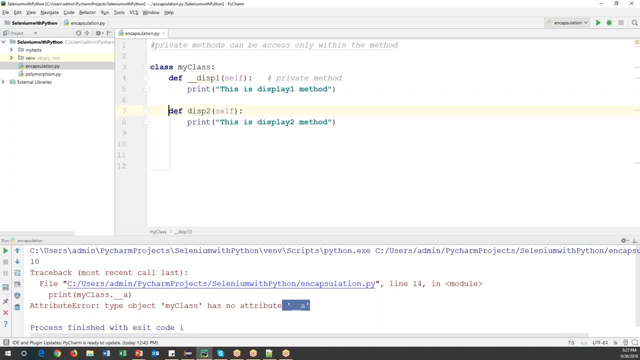 one more method, Which Is this method right? So I already have displayed to in this method itself. I will call the private method. I will call this private method. how to call this private method from here. how to call this private method here: 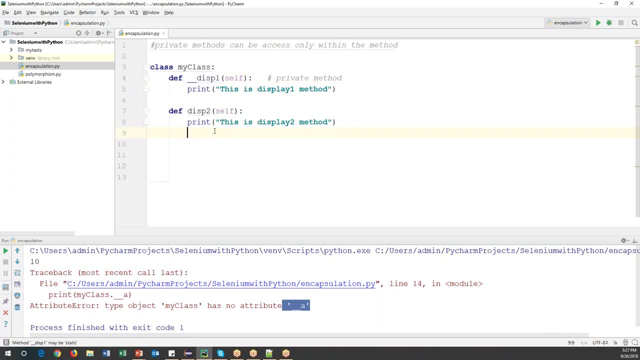 So this method is belongs to class right. how we can access this class method? again, We have to use selfie keyword. Remember this: always, whenever we want to access any variable which is under class, We have to specify the self. So always we have to refer class variables and class methods with the self keyword. 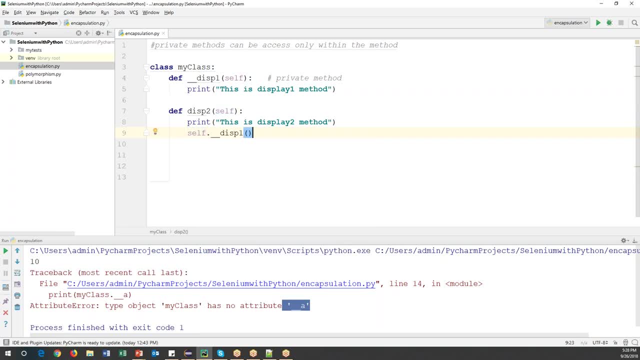 So self dot underscore, underscore, display one. So this is how we need to call. So the same method I am calling from the second method. Okay, so both the methods are in the same class. So display to method easily can access the first method. 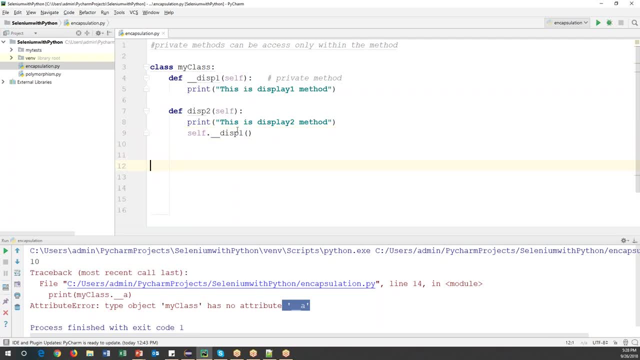 Okay, now I call this method. now come out from the class. So which class I need to execute now? I need to call the first method. I cannot call. I can still call the first method by using an object. Let me just show you Here. 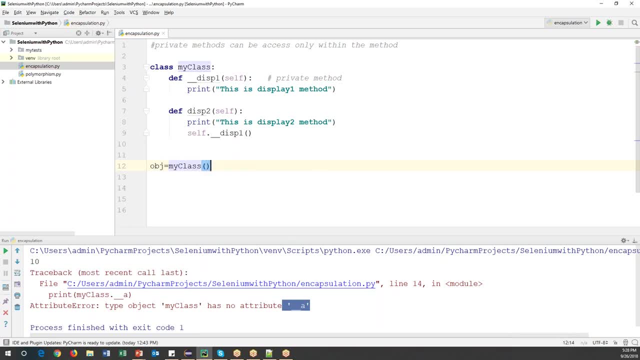 I will create an object for my class- Okay, my class. now let's see OBJ dot. when I say OBJ dot can be called display one method, here There is a private method. Yes, we can still call display one method. Can we call display one method? 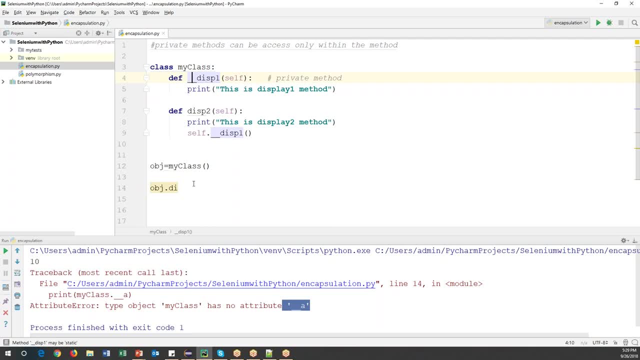 So this is a private method, right? So even though it is a private method, can be called from the outside object we created, right? So through object can be called this private method. Let's see So: OBJ dot- underscore, underscore, right? So this is the one method, right? 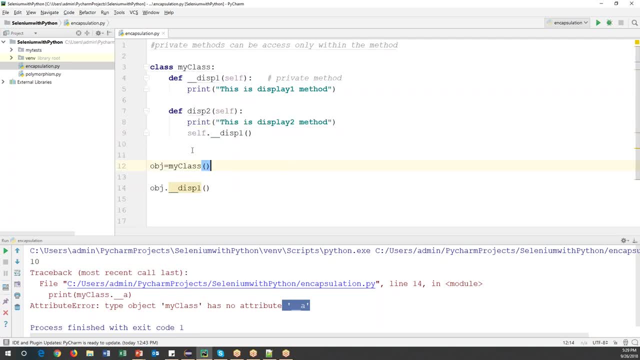 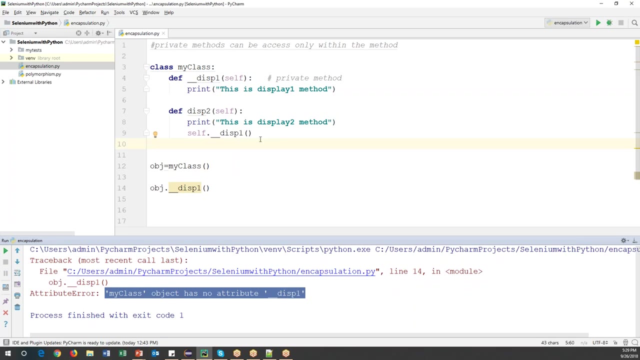 So I'll just call So: OBJ dot- underscore- underscore this one. this is a private method. I'm just calling like this: underscore- underscore. this method can be called like this: let's run this code and see: is giving error: my class object: no attribute- underscore this one. 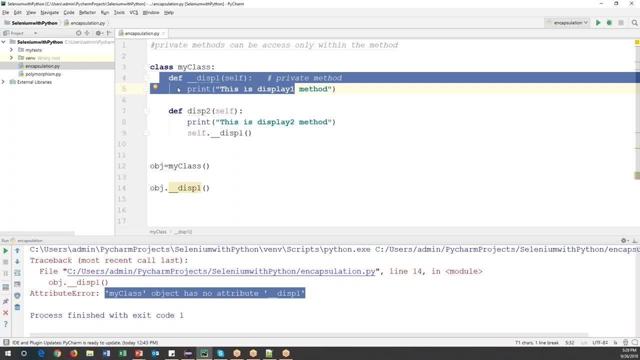 So we cannot access this directly from the object itself. Okay, Okay, So because this is a completely private within the class only we can access, So here object is itself is outside of the class, right, We cannot access this, but can we access the dispute to method? 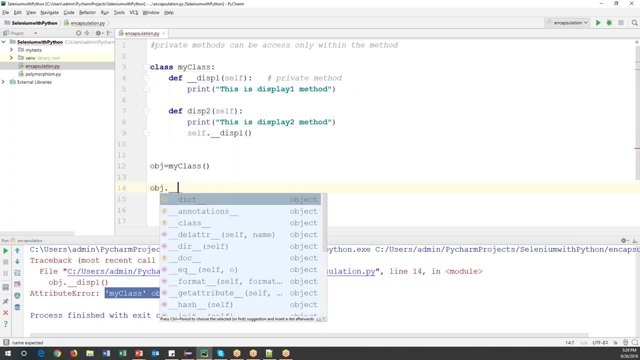 Yes, we can access. So now, when I access this to method, what happens this particular method? So when I access this particular right? so now what happens? OBJ, I just created for my class object. I'm just calling the dispute to method. Okay, So this to method. 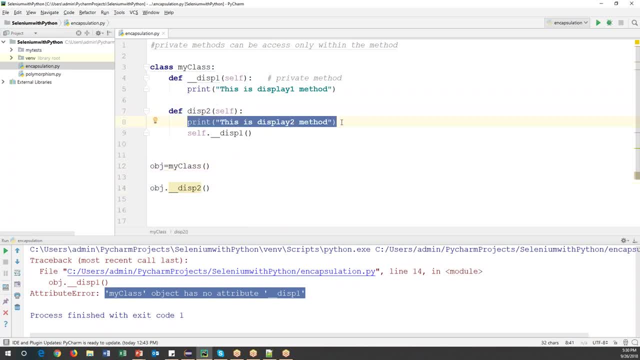 So what happens now? this to method will be called here. first it will print this message and after that, internally it will call this to one method. Okay, this to can call this method right. this one, because this tool and this to one. both are there in the same class. 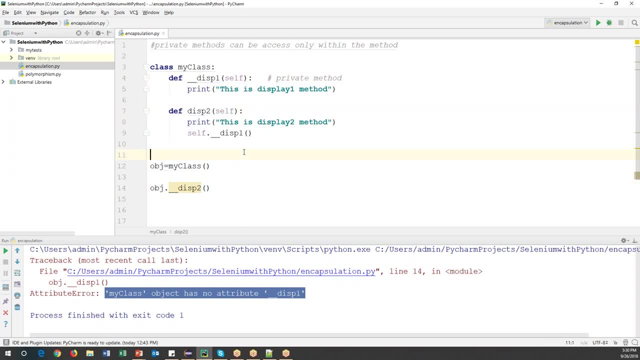 So this one is a private, can be accessed within the dispute itself. So when I run this again, we are getting issue attribute. my class object has no attribute. underscore this one. Let's see what is the issue here. Oh sorry, here I have made an underscore and this is wrong because this to is not a private. 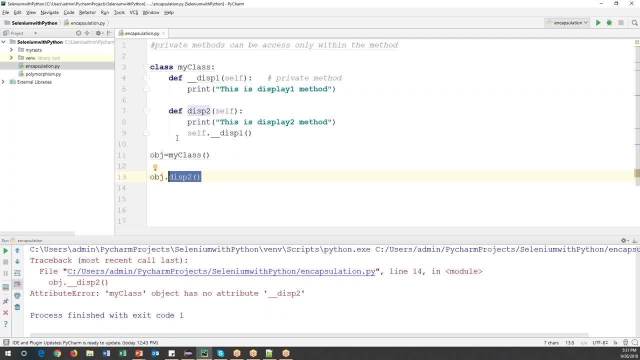 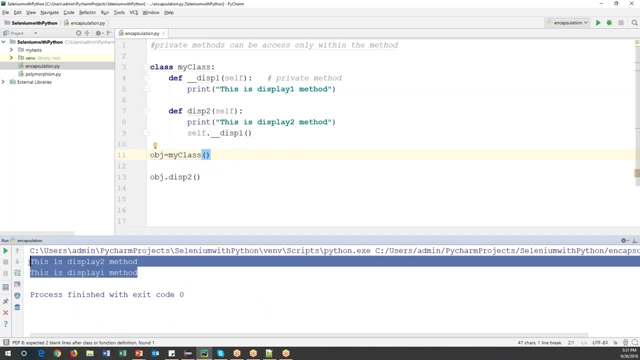 method right. So this to is not normal method is a normal method, So we can directly call this to dispute to from this object. So now let's run this. Now we can see we are getting to outputs. So when I call this to dispute to method first, it will call here: 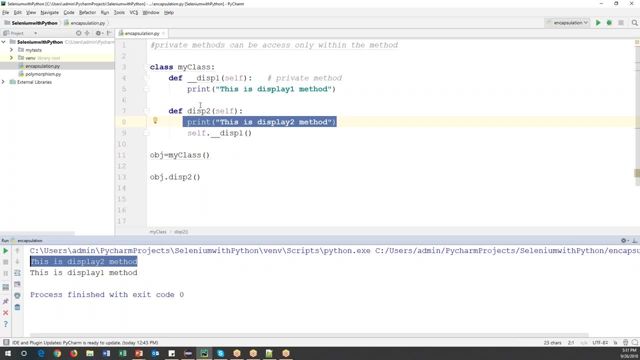 So first it will print dispute to method. So it is printed here and again in the dispute to method. internally we call display one method. So it will go up and call this. It is possible here because this to one is a private method can be accessed within the. 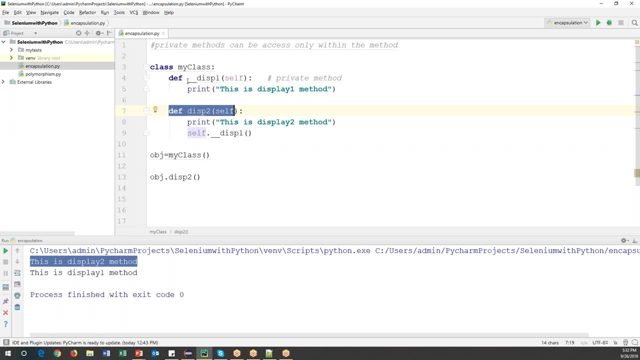 dispute itself again because this to is also part of the same class. but outside of the class we can have access. outside of the class we can add a, as I said before, OBJ dot underscore, underscore, and this to one is not possible because outside of the class we are calling. 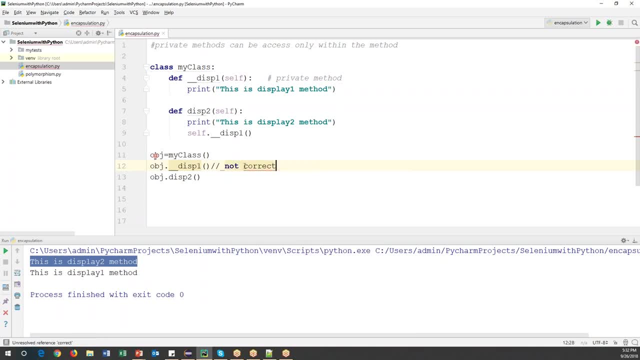 here. This is not correct. This is a not correct one, So this is a. this is not correct, but still we can call this. Okay, This is, we can call this. So this is how you can create a private methods, So private, private methods on private variables. 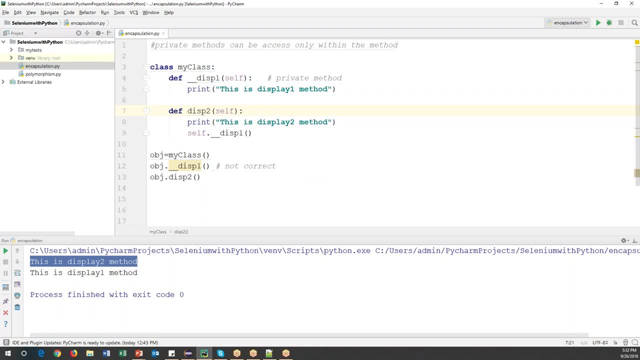 So we have seen two examples. So one is for a private variables can be accessed only within the class. and also I have shown you private methods. Those methods also can be accessed only within the class, only within the class. Now I'll show you one more example. 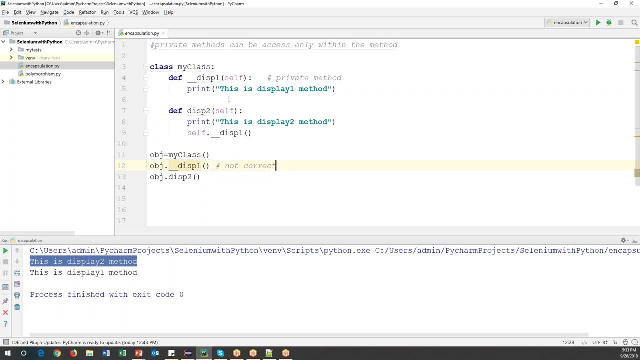 So in the, in these two examples, What we understood is we have come to one conclusion: that private variables and private methods We cannot directly access outside of the class, only within the class: variable taxes. but there is one more scenario where we can still access class variables, private variables, by 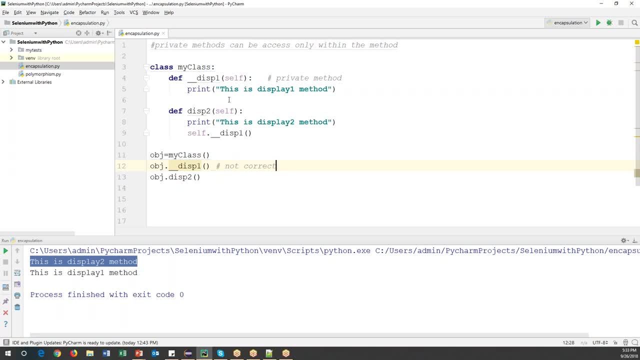 using some methods. Okay, I'll show you alternative way of accessing the private variables. So let me just create one more example. So what I'm saying is: We can access, we can access private variables outside of the class if class outside of the 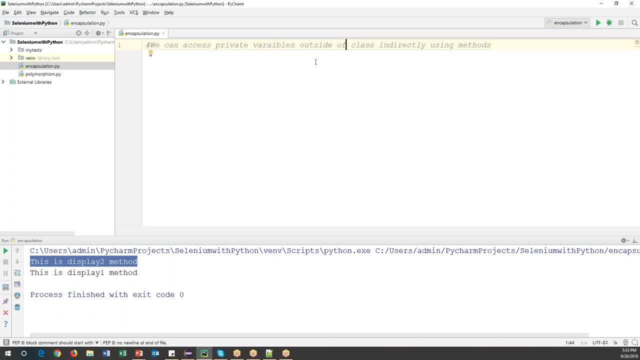 class right outside of the class, indirectly using methods. indirectly using method, we can access private variables outside of the class indirectly. It is not direct taxes, I'm saying okay, but using some methods we can access. let us see how we can do that. I will create one class called as a, my class, my class and inside the class. 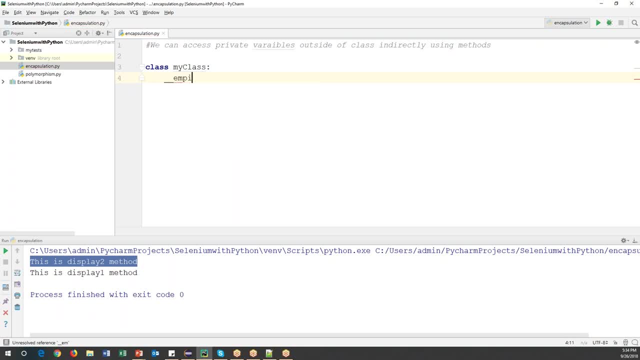 I will create. I will create a one private variable. I will name is as a EMP ID and by default, I will give one value to this. This is a EMP ID empire. along with very cool, I will also create one method display: get EMP ID. get EMP ID to say, get EMP ID is a my 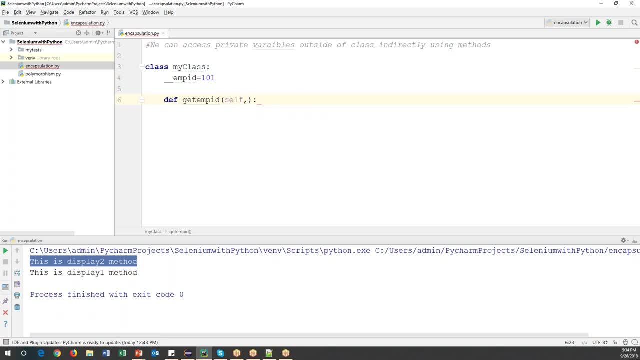 method and self, and this method will take EMP ID from outside, will pass this ID later and inside, what I will do is, whatever ID are getting, I will. I will assign this ID to the existing variable. Okay, how we can do that, how we can access this variable inside, the method can be accessed. 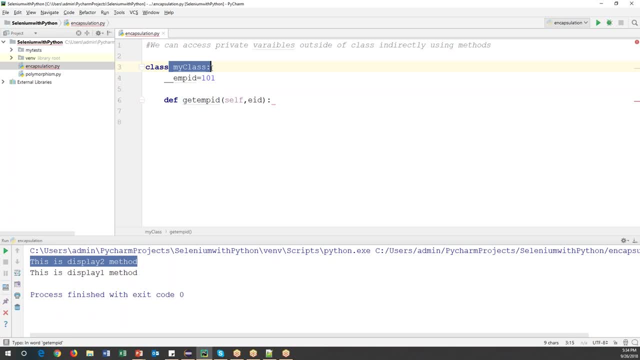 right, because this is a private variable. This method is also part of the same class, so we can access this variable directly. how we can access? by using self the keyboard, because this variable is belongs to the class. So always class variables We can access by using self the keyword so that I can say self dot. underscore, underscore. 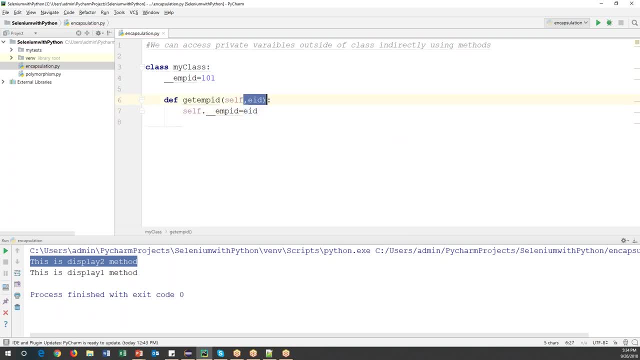 EMP ID is equal to EID. I'm assigning Whatever value You are getting, I'm assigning this. So this is a one method I created. now I will create one more method: dev okay, and this display EMP ID. for displaying EMP ID and. 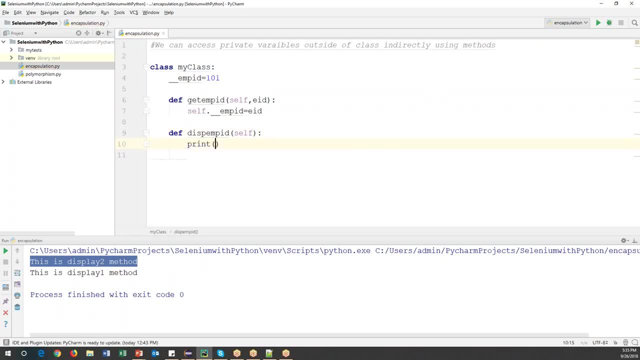 creating one more method. So here I will just print the EMP ID, Let's say print how we can print this value. EMP ID again: self right, self, dot, underscore, underscore: EMP ID. So one method will get the EMP ID from the outside And it will reassign the value, whatever value are already existed. 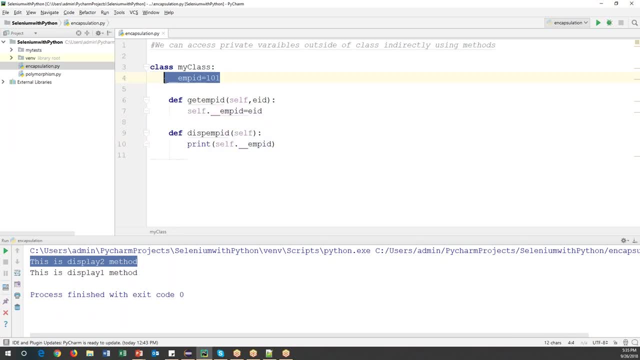 It will reassign the value and the other method will print the value of EMP ID. Okay, Now we can see the before examples I have shown you. we cannot access this private variables outside of the class. outside of the class, We cannot access it, but still now I can access this variable value outside of the class through. 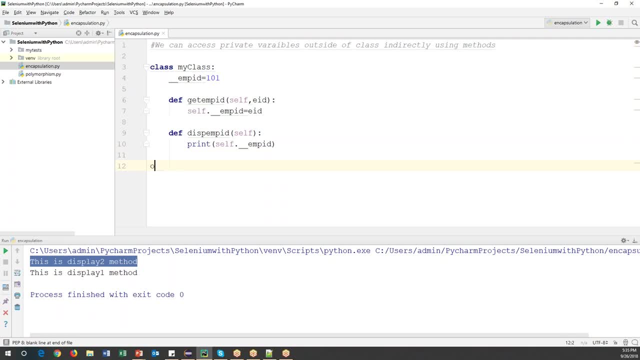 objects. So let me just show you how we can do that. I will create an object for my class. I will create an object for my class. So for this object, using this object variable, I can call this method right: get EMP ID. because 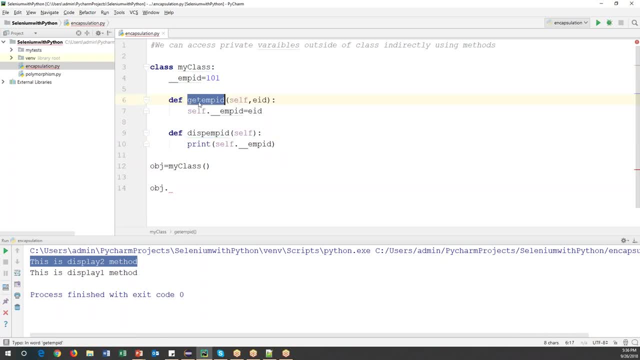 this is a, not private. both are normal methods, not private. So get EMP method ID, get EMP ID. I can call right and I will just pass EMP ID as a 102 now. Now, what happens here? What happens here when you say: obj dot, get EMP ID, or okay? 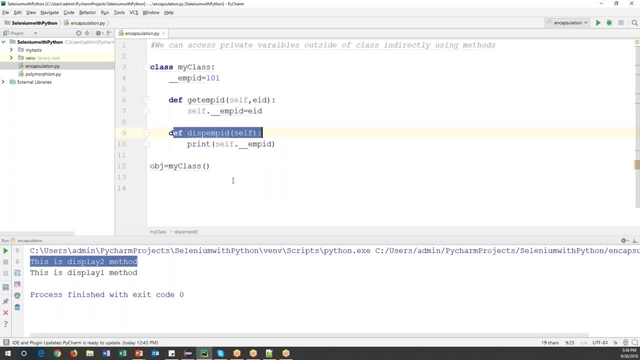 So we will see this in a related. For now, What I can do is I will just call EMP ID- display EMP ID as a obj dot. obj dot- display EMP ID. Now what happens? So when I say obj dot- display EMP ID from this object, it will call this method right. 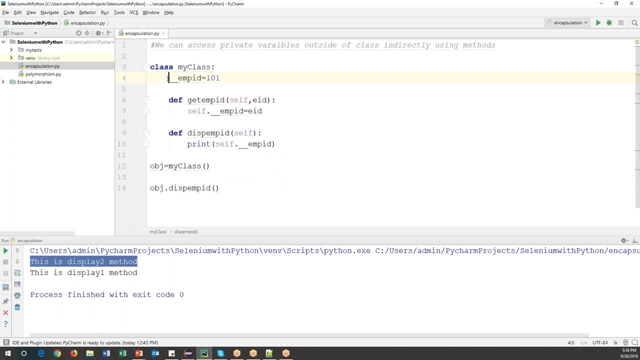 the second method will be called. what the second method will do: it will print the value of EMP ID. It will print the value of EMP ID, right, and I run this. it will give you one, zero one. So what I have done here, I'm indirectly access this variable outside. 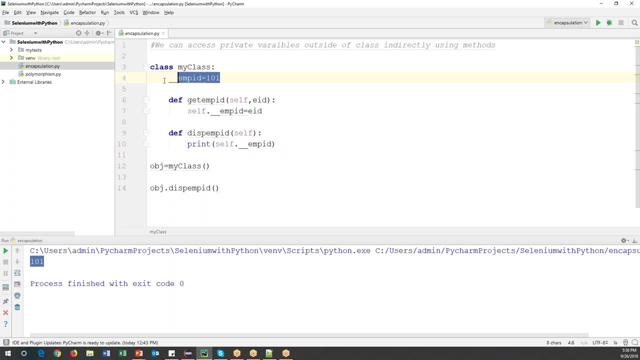 Of the class right. so I have indirectly access this private variable outside of the class. How am I accessed through this method, even though if you have an object, we can directly, if you don't have this method, we can- that we cannot directly access this, but to access. 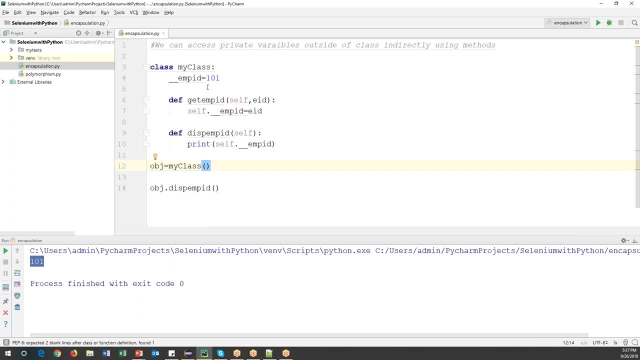 this. I have just created one method and this method internal can access because this is a private variable. This method is we again belongs to the same class, So this method can access directly this variable. Okay, But this method I cannot call from the outside of the class through object. 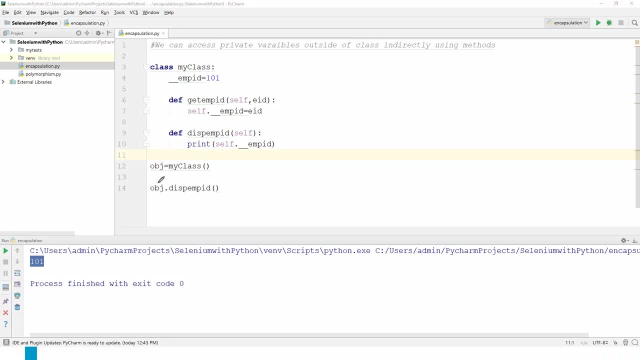 All right. So now what happens is? it happens like this: So first we have called this empty right. So this will call this method: first: display EMP ID self. it will call now internally: what is what I'm saying here? I'm referring this variable here, right? 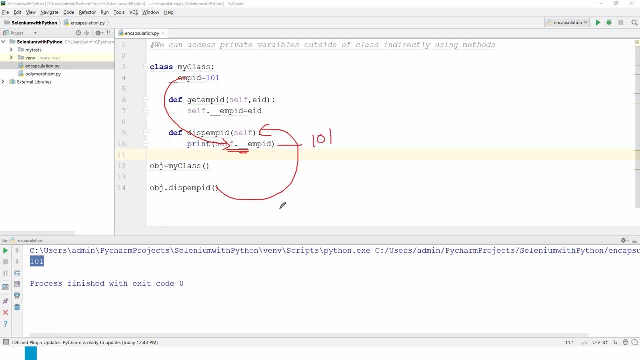 So now it is printed exactly one, zero one. So this is how it will work. Okay, So this is indirect process. We are not directly accessing this variable. We are going to calling the method and method will call this variable. All right, 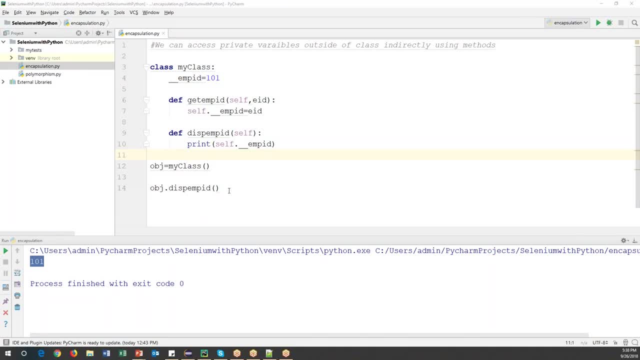 So this is how it will run. Now I'll show you one more. suppose even a pass some value here. So before displaying the value, I will also call this get EMP ID method. by using OBJ want to change the value of EMP ID now, even though it is a private variable, I can change that. 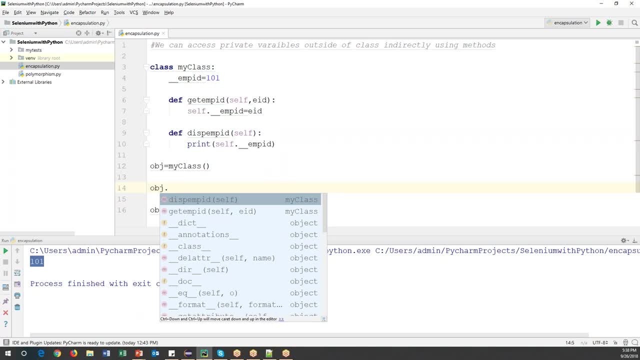 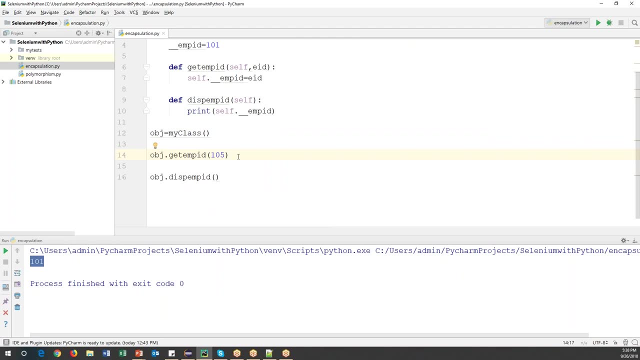 value indirectly from outside of the class. So OBJ dot- get EMP ID. I will just make it as a onesie. So now what happens? now what happens? this method- get EMP ID method- directly call this one and whatever value we are assigned, the value will be assigned to the key ID. 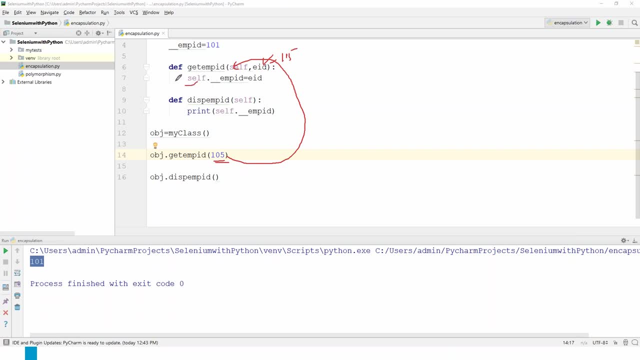 So it will become one zero five. now, internally, what happens now? this will refer the class variable right self dot EMP ID referring the class variable. that new ID will be assigned to this one. Now what happens is the class variable value default is one zero one. 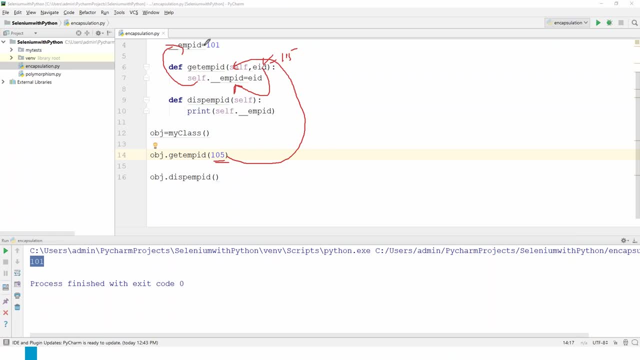 Now we have passed a new value, The new value will be assigned, That's, into this variable. now, current value of EMP ID is one zero five. Okay, becomes one zero five. now what happened now? immediately call the print method. So it will call this method again. 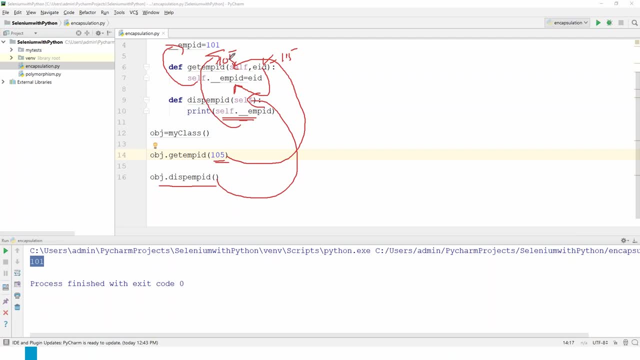 It will refer the same class variable. Now, currently the class variable EMP ID value is one zero five, So now we will get the one zero five. Okay, so this is how it will execute now let us see. Let me just execute this and see: run as: